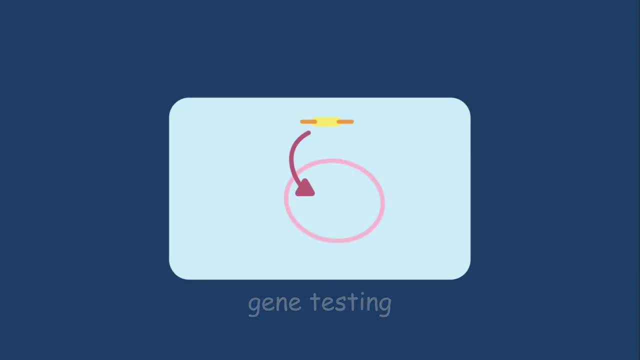 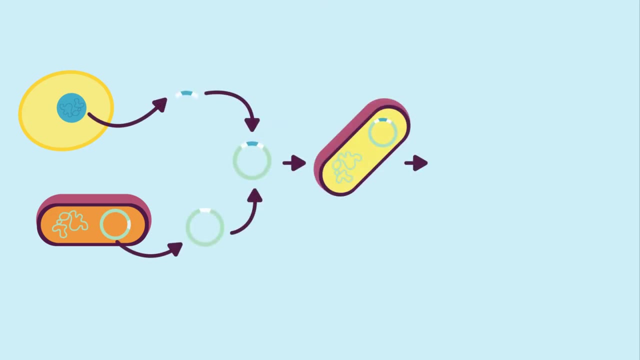 genetic engineering: vaccines, gene therapy and gene testing. You may know how human genes are transferred to host bacterial cells, which then produce large amounts of substances humans require, such as hormones like insulin. This is a form of gene technology called genetic engineering. GM crops are also an example of genetic engineering, whereby inserting genes 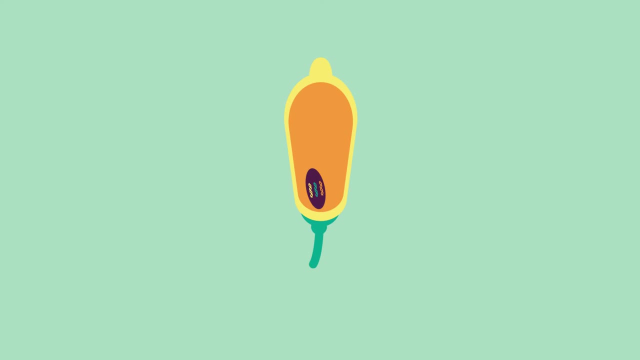 from one organism into another can give a crop plant an added advantage, such as increased nutritional value, resistance to pests, resistance to drought, and resistance to fungi and bacteria that cause rotting and decay, thus making the crop food last longer. All these 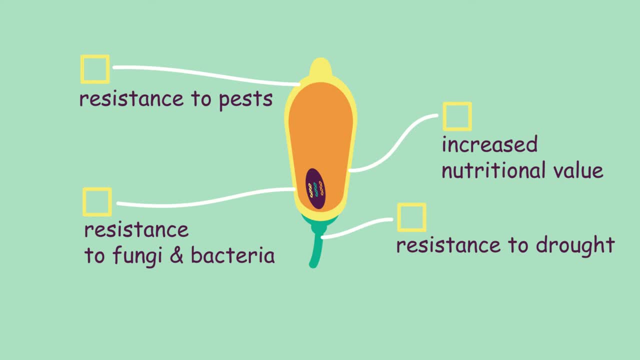 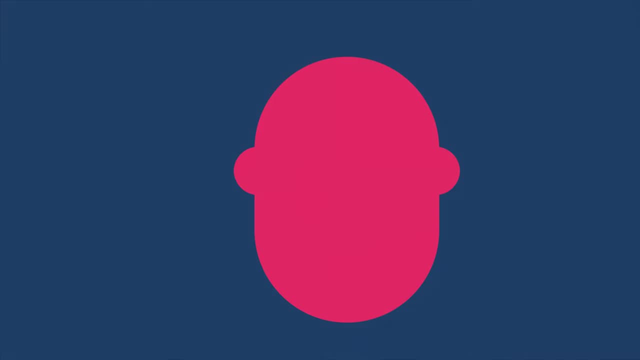 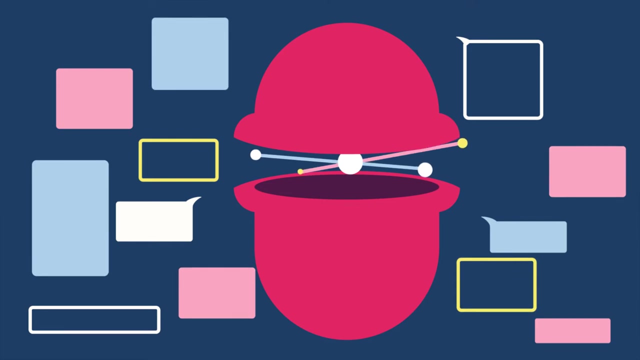 advantages increase food security, which is very important and beneficial given the increase in the human population. Let's now discover some other examples of gene technology. As you find out more about these gene technologies, think about ethical considerations involved with the application of these technologies. Vaccines prevent hundreds of potentially fatal diseases. 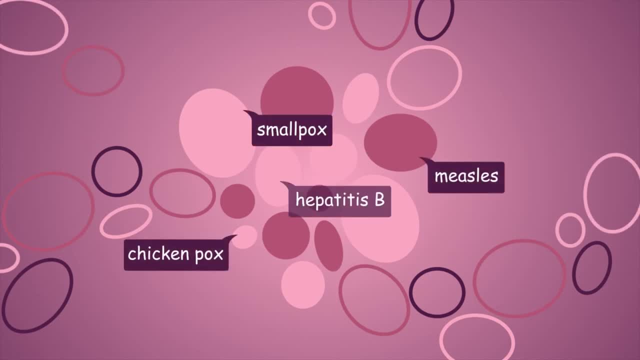 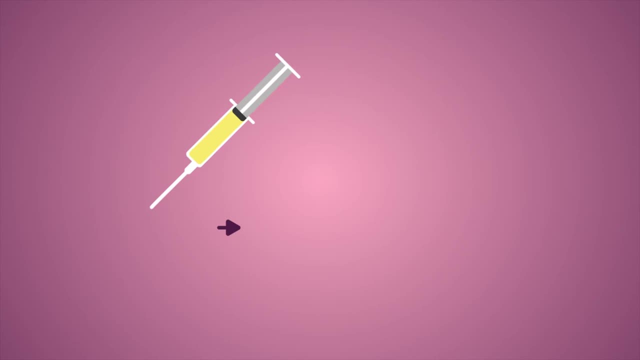 such as measles, smallpox, chickenpox, hepatitis B, tuberculosis and influenza. So how do vaccines work? Vaccines contain inactive particles of viral coats, which contain proteins called antigens, specific to the virus itself When the vaccine is injected. 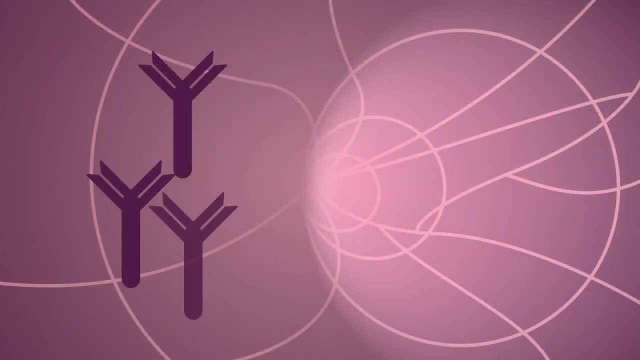 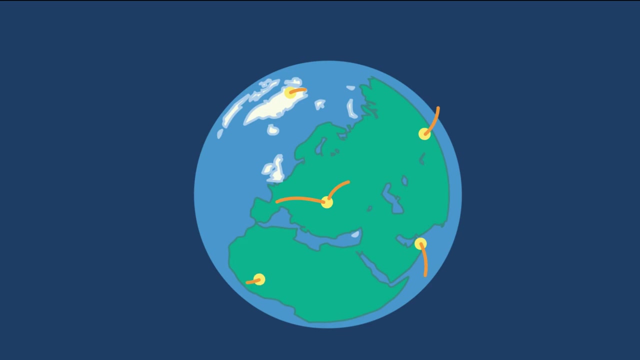 into the body, the immune system immediately produces antibodies against the antibodies, which are the antigen proteins on these viral particles. If the person comes into contact with the actual virus, the body is already prepared to fight the infection with its antibodies. This all sounds great. However, there are problems associated with the distribution of vaccines. 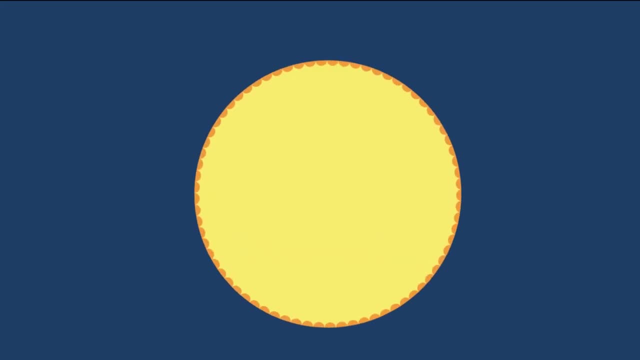 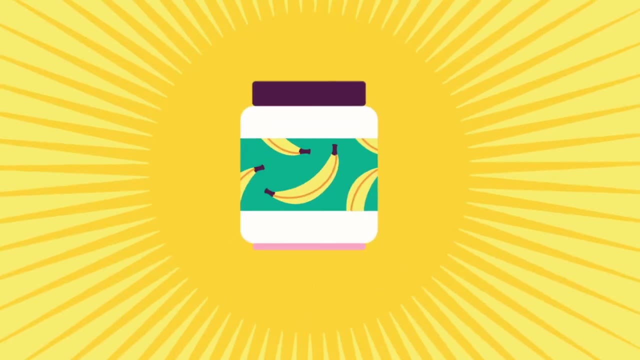 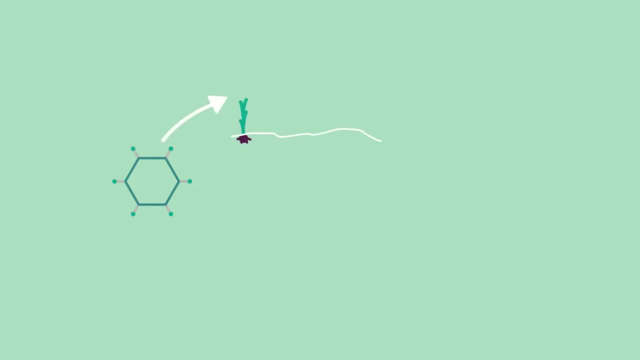 especially in developing countries. Vaccines are expensive and need to be stored at low temperatures, as they will be destroyed by heat. The solution Enter edible vaccines. Scientists can inject an antigen-based form of a virus into a plant, such as a young banana plant, As the plant grows. 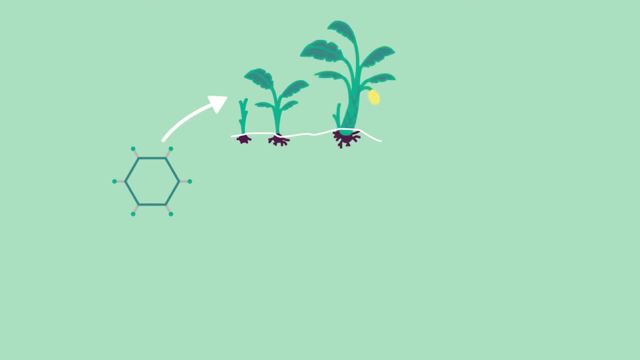 its cells produce the virus proteins, but not the infectious part of the virus. When people eat a genetically engineered banana which is full of virus protein, their immune systems build up antibodies to fight the disease, just like a traditional vaccine. Another form of gene. 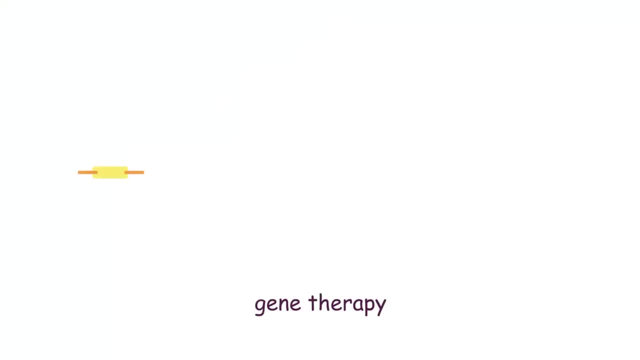 technology is called gene therapy. Gene therapy is when DNA is introduced into a patient to treat a genetic disease. The gene therapy is when the DNA is introduced into a patient to treat a genetic disease If a particular gene has mutated causing a genetic disorder, such as cystic fibrosis. 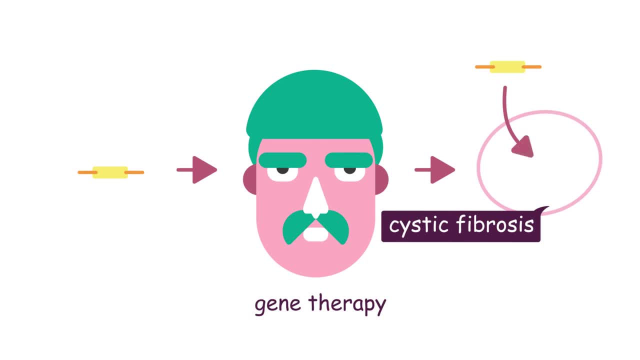 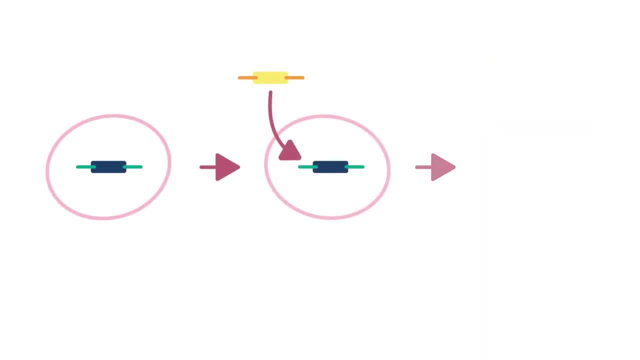 new DNA containing a functioning gene is introduced to correct the effects of the disease-causing mutation. Gene therapy can also be used to block or switch off a gene that is causing cells to malfunction. For example, in some forms of cancer, gene therapy can even be used to kill cells that. 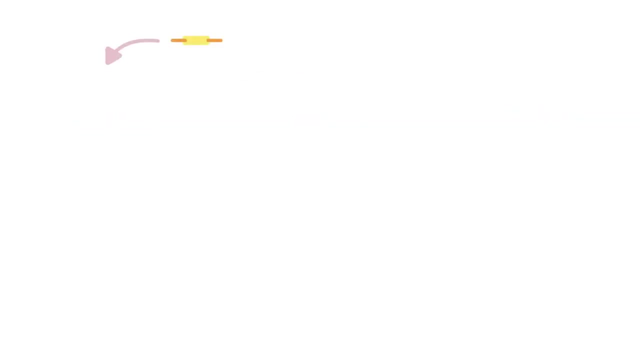 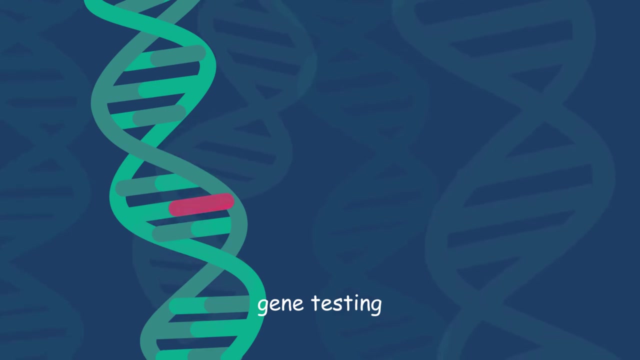 are diseased. In gene therapy, the new genes are introduced into the cells via a vector, which is a non harmful virus that carries the gene into the patient's cells directly. Genetic testing is a form of gene technology that is done if a genetic disorder is suspected, If you have symptoms of a. 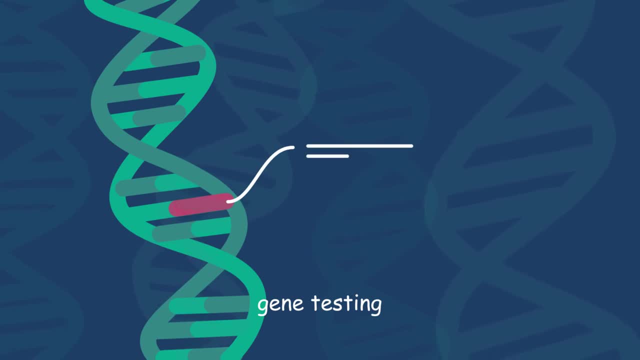 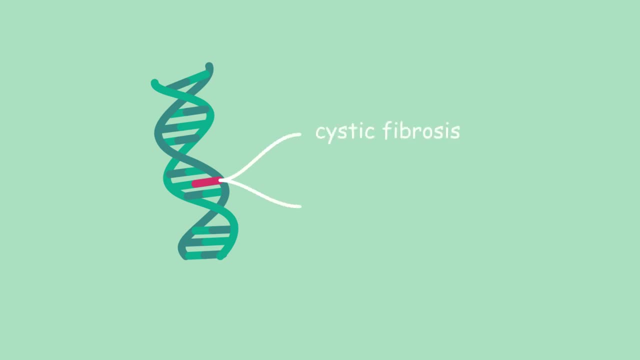 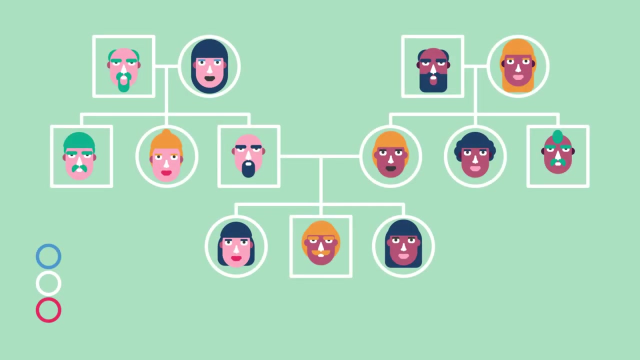 genetic disease. genetic testing can confirm if you have the suspected disorder. For example, genetic testing may be used to confirm a diagnosis of cystic fibrosis or Huntington's disease. Genetic testing can also be done if you have a family history of genetic conditions. 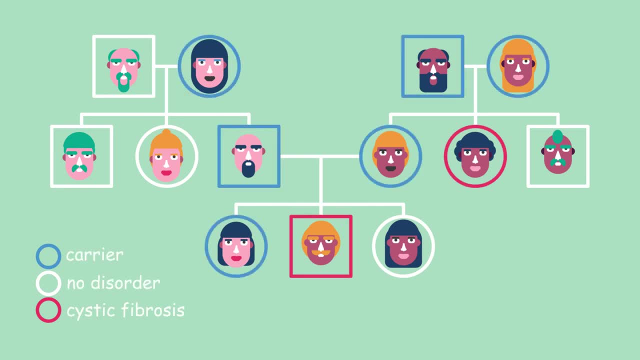 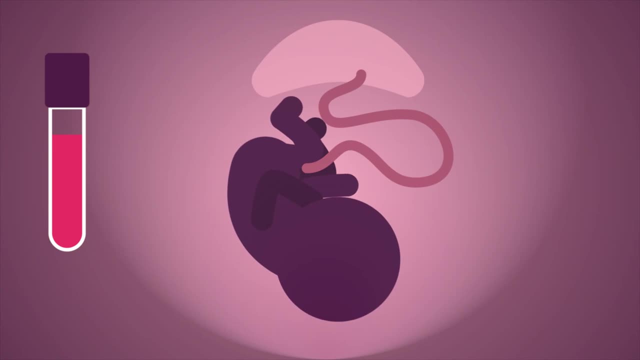 sickle cell anemia or cystic fibrosis, or you're in an ethnic group that has a high risk of a specific genetic disorder. If you're pregnant, tests can detect some types of abnormalities in your baby's genes: Down syndrome and trisomy 18. 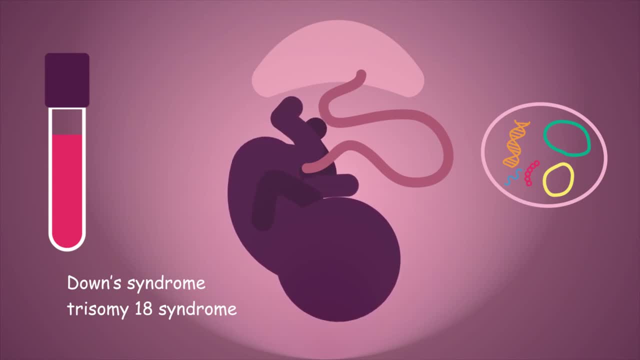 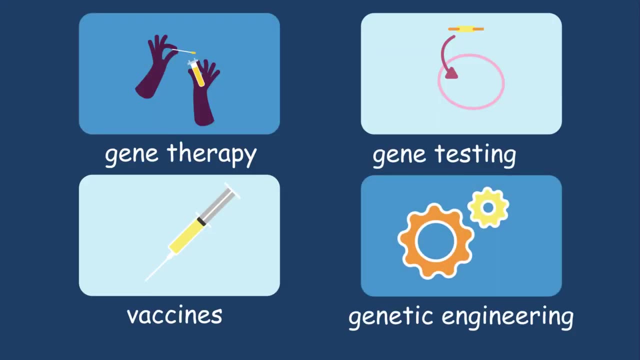 syndrome are two genetic disorders that are often screened for as part of prenatal genetic testing. All forms of gene technology exist to benefit humans by preventing and curing diseases and ensuring food security. However, there are potential issues that exist with any form of genetic modification. Here are 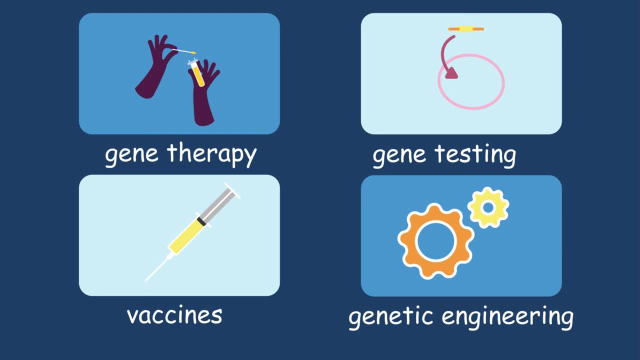 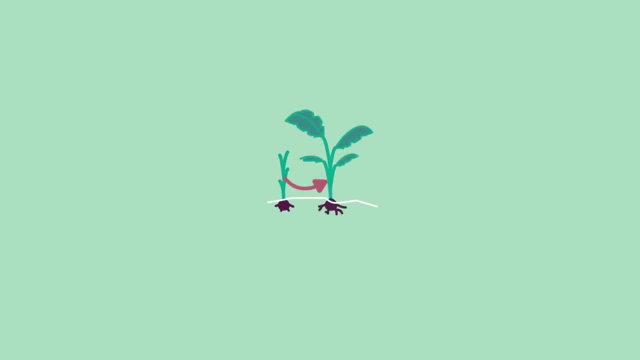 some questions to get you thinking about the ethics of gene technology. What is right and what is not ethical In genetic engineering? could inserted genes spread to non-GM plants in the wild, thus endangering biodiversity? Could farmers be forced to buy expensive genetically engineered seed when they have? 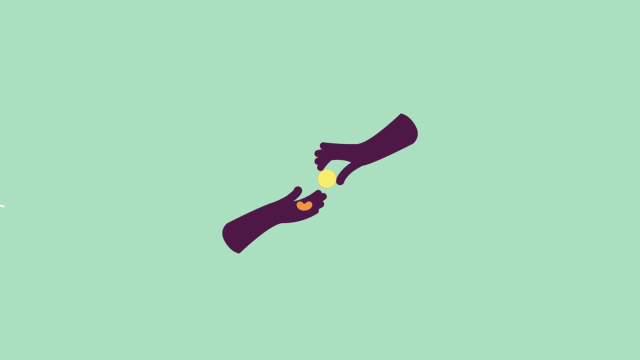 traditionally kept some seed to plant the next season. Is it moral to modify genomes? Some people believe that it is ethically wrong to move genes between different species. In terms of gene therapy, who decides which conditions require treatment? It could be tempting to also cure conditions like baldness and obesity. This would be improvement, not treatment. The technology could be misused In the future. superhuman soldiers with certain physical and intellectual characteristics could be created. These individuals would have no say in this. Would this be ethical? People believe it is not ethical to interfere with genes and individual species particularly.